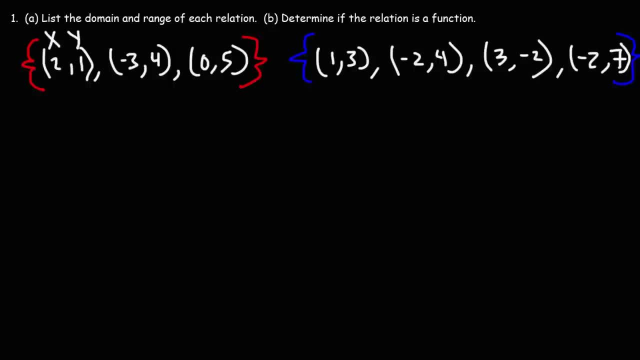 The x values is associated with the domain of the relation. The y values is associated with the range of the relation. So now let's focus on part a list: the domain and range of each relation. So let's start with the domain. So what we're going to do is we're going to make 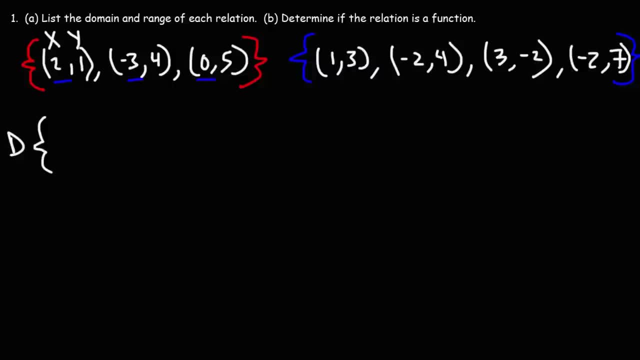 a list of all of the x values and I'm going to write it in ascendant order. So first we have negative three and then zero and two. Now let's write the range of that relation. So we're going to focus on the y values and it's already listed in ascendant order. 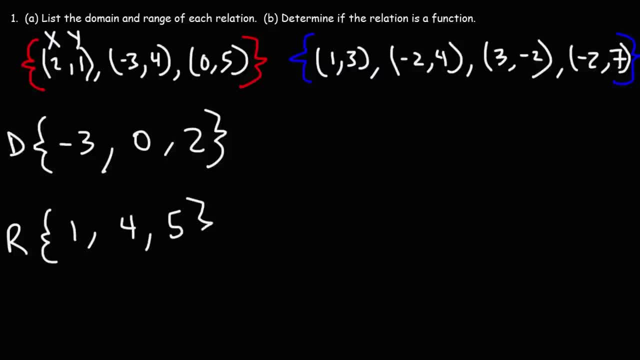 So one, four and five. Now let's do the same thing for the other relation. So let's write out the domain. So the lowest x value is negative two, Next is one and then three. Now let's write out the range of that relation. The lowest y value is negative two. And then it's three, four and five. So let's write out the range of that relation. The lowest y value is negative two, And then it's three, four and five. Next it's negative two, And then it's three, four and five. 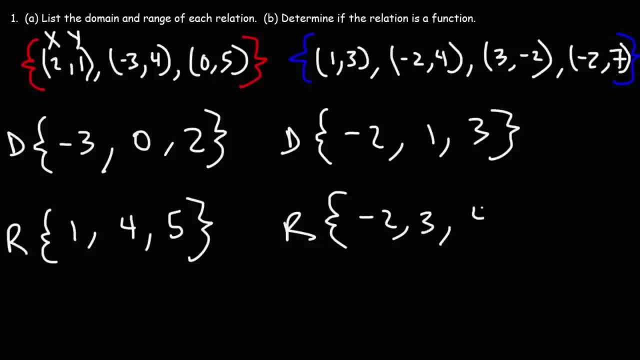 Next is negative two, And then theELY value is negative two. So now we've have destroyed the pretty important好吃. the first thing is to write in ascendant order, So that's how you can write the domain and range of each relation. 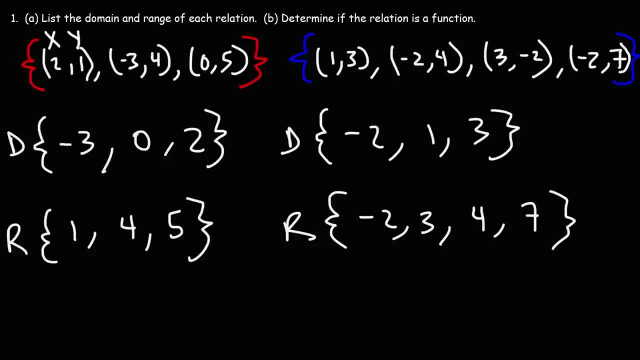 Now, how can we determine if the relation is a function? In order for the relation to be a function, every input value must have only one output value. If a input value corresponds to two or more output values, the distance created between the output valuesilated is greater than the the values of the other relation. 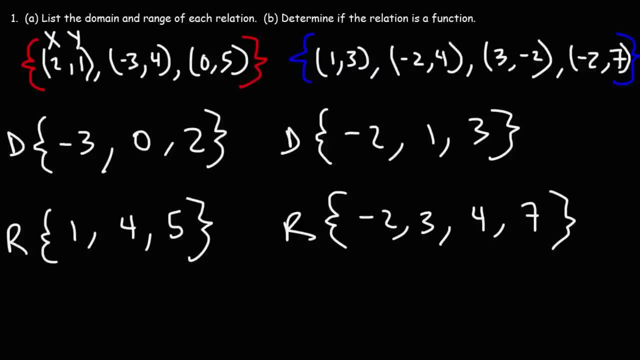 In order for the relation to be a function, you must see all of the secrets within this value: output values. that relation is not a function. now let's focus on the first relation. so we have the ordered pair 2: 1. the input value is 2. the output value is: 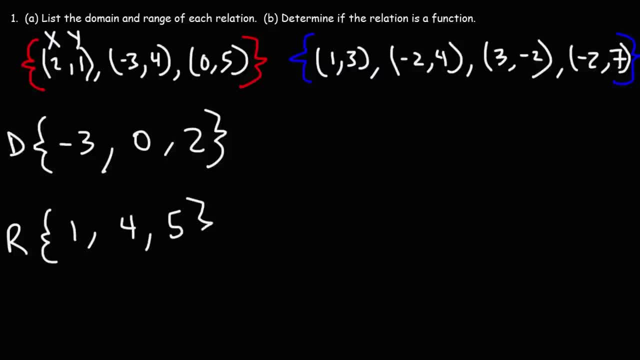 So one, four and five. Now let's do the same thing for the other relation. So let's write out the domain. So the lowest x value is negative two, Next is one and then three. Now let's write out the range of that relation. The lowest y value is negative two. 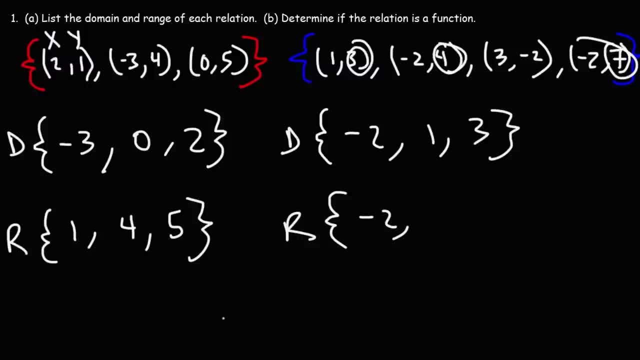 And then it's three, four and five. Three, four and seven. So that's how you can write out the domain and range of each relation. Now how can we determine if the relation is a function? In order for the relation to be a function, every input value must have only one output value. 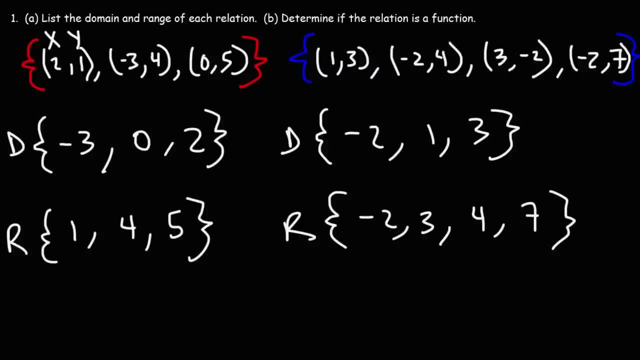 If an input value corresponds to two or more output values, then the output value must be negative one output values. that relation is not a function. now let's focus on the first relation. so we have the ordered pair 2: 1. the input value is 2, the output value is: 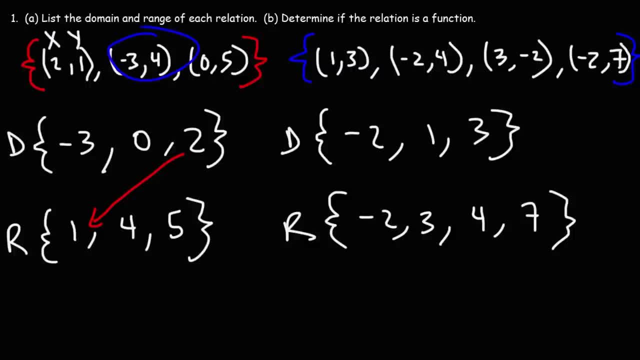 1 and then negative 3, 4. so negative 3 corresponds to 4 and then 0 corresponds to 5. so for the first relation we can see that for every input value there's only one output value. now let's focus on the second relation. so we have the. 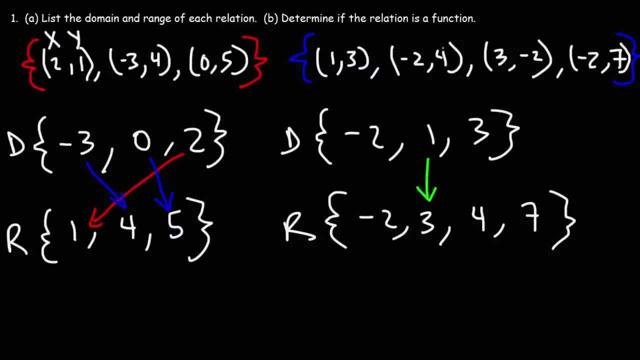 ordered: pair 1, comma 3. next is negative 2, 4, and then it's 3, negative 2 and then finally negative 2, 7. so for the second relation, notice that negative 2 corresponds to two different output values. now that's a problem if you put in an input value of negative 2. 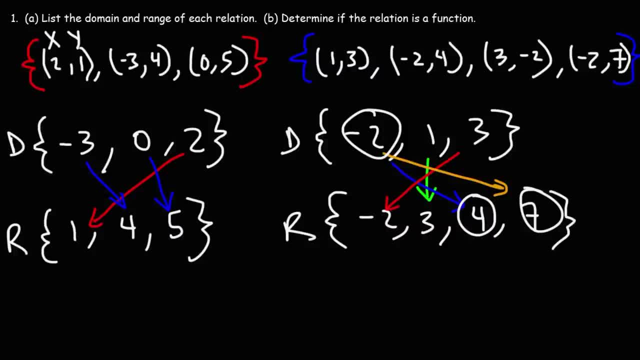 should the output be 4 or 7? so whenever you have that situation, you know that relation is not a function. the first one is a function. every input value corresponds to a function, to an output value, just one output value. so a quick way to look at a. 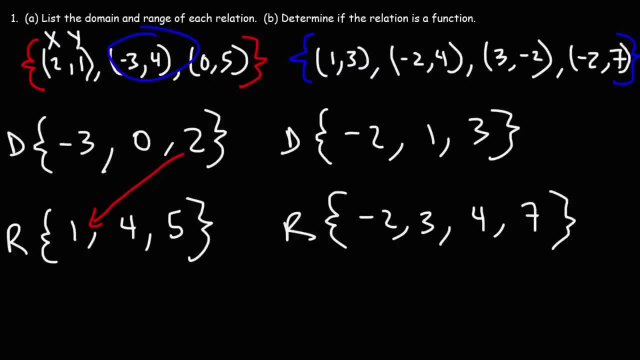 1 and then negative 3, 4. so negative 3 corresponds to 4 and then 0 corresponds to 5. so for the first relation we can see that for every input value there's only one output value. now let's focus on the second relation. so we have the. 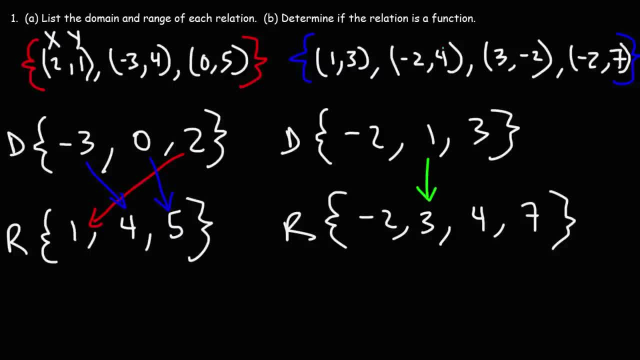 ordered: pair 1, comma 3. next is negative 2, 4, and then it's 3, negative 2 and then finally negative 2, 7. so for the second relation, notice that negative 2 corresponds to two different output values. now that's a problem if you put in an input value of negative 2. 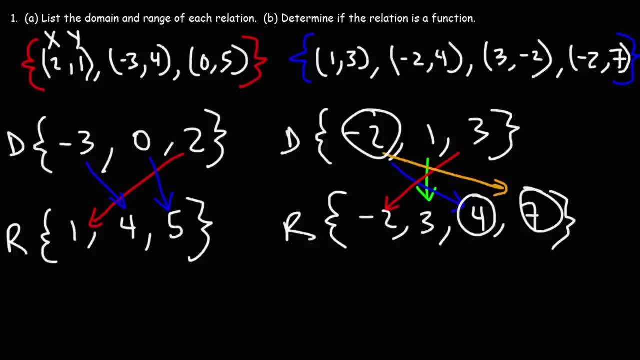 should the output be 4 or 7? so whenever you have that situation, you know that relation is not a function. the first one is a function. every input value corresponds to a function, to an output value, just one output value. so a quick way to look at a. 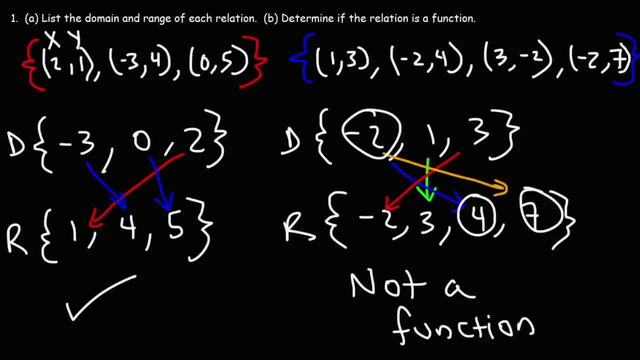 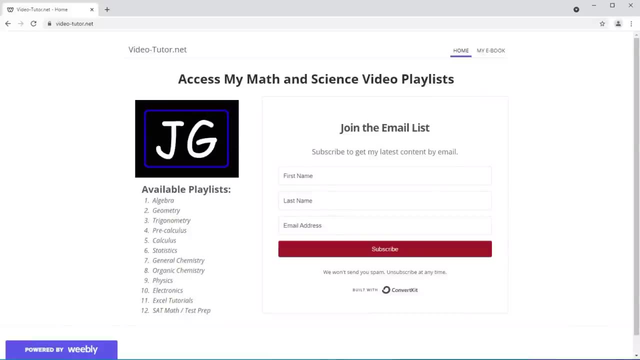 relation to see if it's, if it's not going to be a function, look for repeating X values. if you see two X values that are the same but correspond to two different Y values, then you know the relation is not a function. I want to take a minute to talk about my website, video-tutornet. it's a very simple. 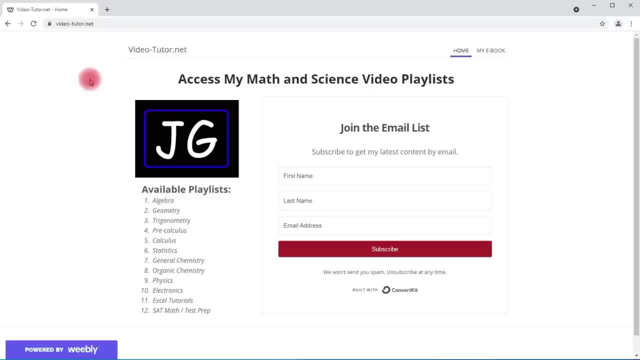 website not too complicated, but for those of you who want to be notified anytime I release specialized content in the form of a video and ebook and article. it could be a digital course or podcasts. if you want to be notified, feel free to join the email list and once you confirm your email, you can get access to a page. 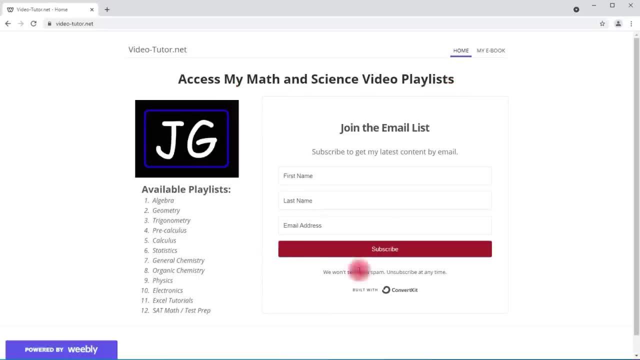 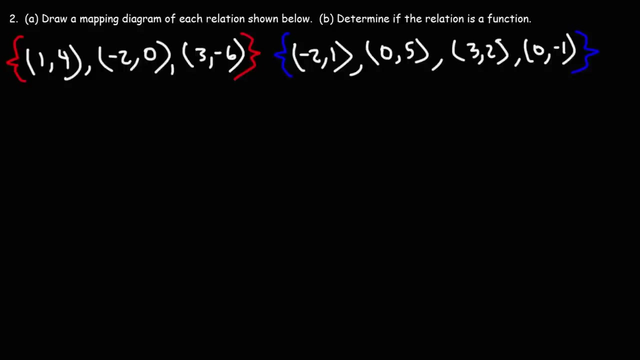 that has all of my playlist listed on it, And this includes my final exam videos and also my test prep videos. So feel free to join the email list when you get a chance. And let's get back to the video. Now let's move on to the next example. 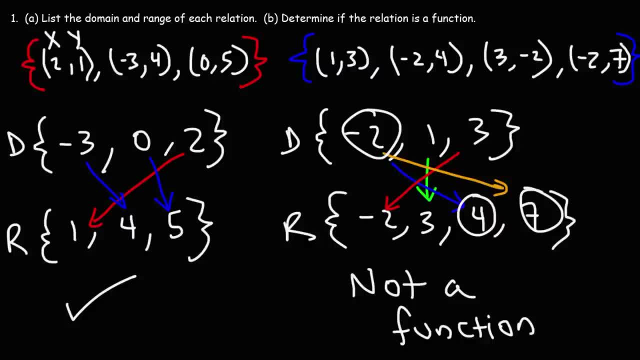 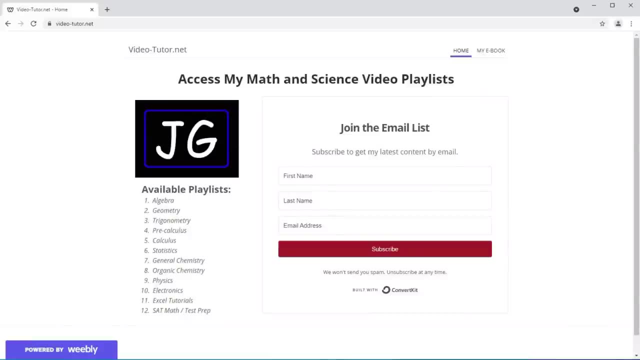 relation to see if it's, if it's not going to be a function, look for repeating X values. if you see two X values that are the same but correspond to two different Y values, then you know the relation is not a function. I want to take a minute to talk about my website, video-tutornet. it's a very simple. 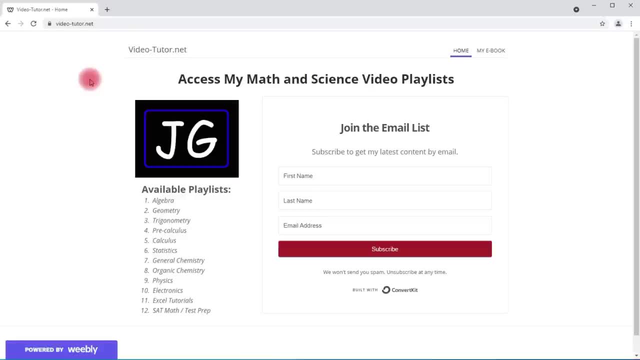 website not too complicated, but for those of you who want to be notified anytime I release specialized content in the form of a video, an e-book, an article. it could be a digital course or podcasts. if you want to be notified, feel free to join the email list and once you confirm your email, you're going to get access to a. 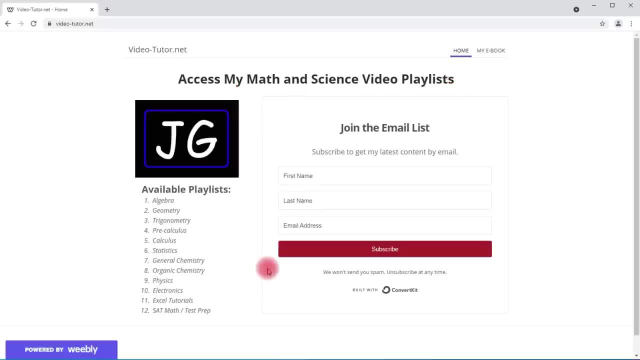 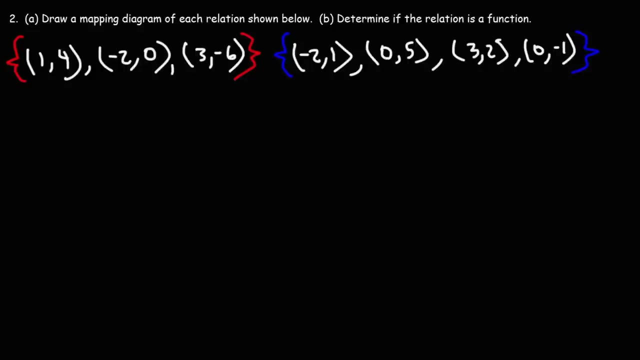 page that has all of my playlists listed on it, and this includes my final exam videos and also my test prep videos. so feel free, join the email list when you get a chance. and let's go back to the video. now. let's move on to the next example. draw a map and diagram of each relation. 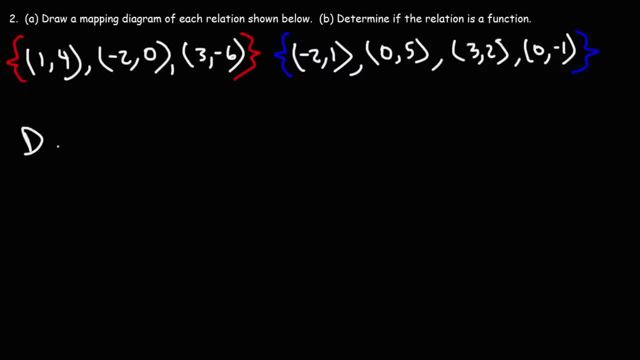 shown below. so let's start with a relation on the left. we're going to map out those three knockouts of the relation for the first position, then we're going to go on to the purposes of the in browser for this test. I just want to take some minutes to do the 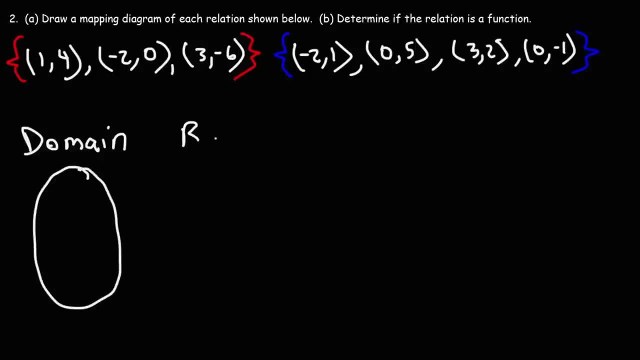 one-to-one inventory to see the ακuma key with you guys. I really needed some out the domain and a range. So for the domain, we have the values negative 2,, 1, and 3.. For the range, we have the y values negative 6,, 0, and 4.. 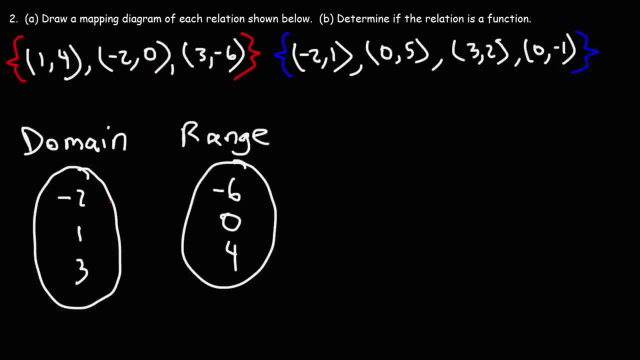 Now negative, 2 corresponds to 0,, 1 corresponds to 4,, 3 corresponds to negative 6.. So for every input value we have the y values. So for the range, we have the y values: negative, 6,, 0, and 4.. 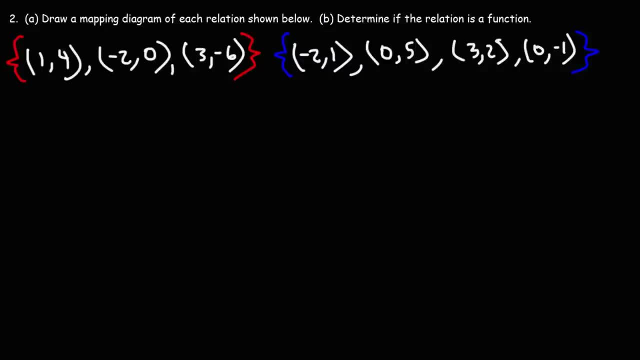 Draw a mapping diagram of each relation shown below. So let's start with the relation on the left. On the left we're going to map out the domain and the range. So for the domain, we have the values negative 2,, 1, and 3.. 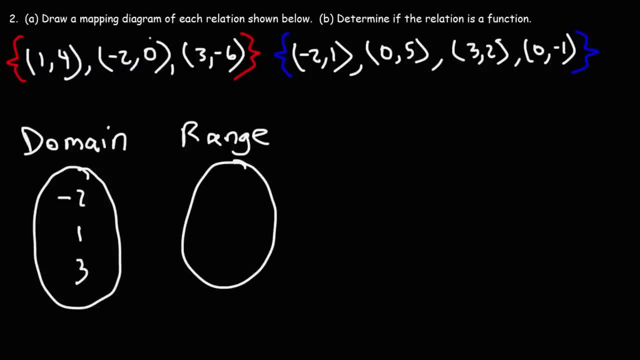 For the range we have the y values negative, 6,, 0, and 4.. Now negative 2 corresponds to 0.. 1 corresponds to 4.. 3 corresponds to negative 6.. So for every input value on the domain side there's one corresponding output value on the range side. 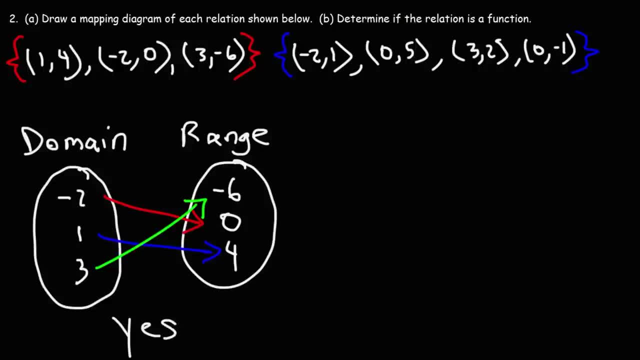 So this is the range And this is a relation. I mean, this relation is a function. So the answer is yes for the first relation. Now let's move on to the second relation. So let's create a mapping diagram as well. 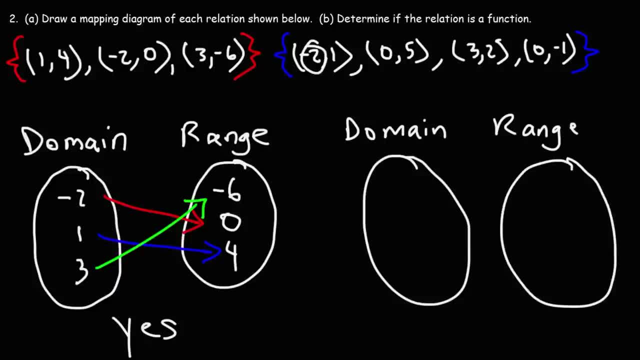 So let's start with the domain. The lowest x value is negative, Negative, 2.. Next we have 0. And then the last one is 3.. Now, looking at the y values, the lowest one is negative, 1.. 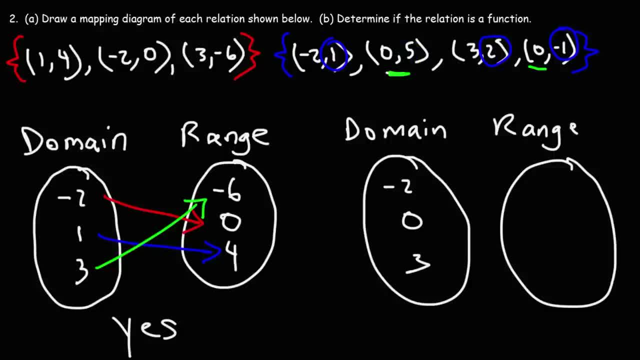 And then it's going to be 1,, 2, and 5.. So negative 2 is negative, 1.. Negative 2 corresponds to positive 1.. 0 corresponds to 5.. 3 corresponds to 2. And 0 corresponds to negative 1.. 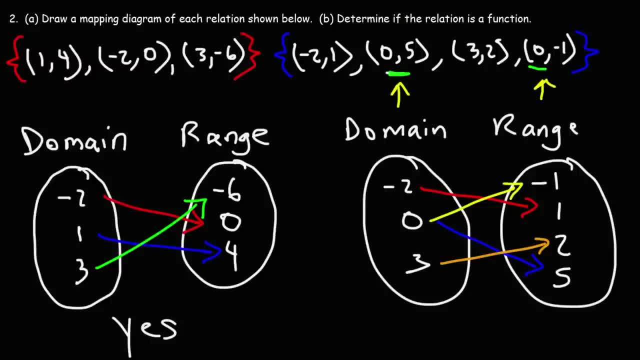 So just by seeing the repeat x values that we see here, we could tell that this is not going to be a function. The two x values have two different y values And you can see 0 points to negative, 1 and 5.. 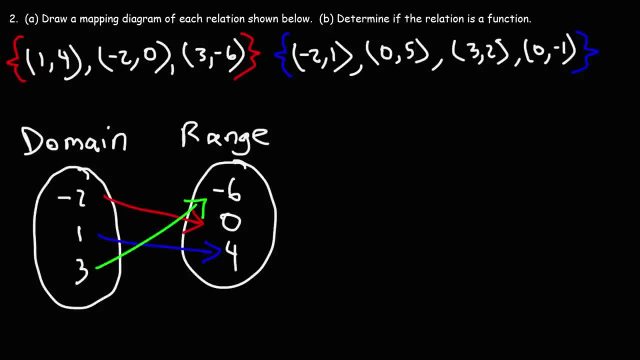 For the output value on the domain side, there's one corresponding output value on the range side. So this is a relation. I mean, this relation is a function. So the answer is yes for the first relation. Now let's move on to the second relation. 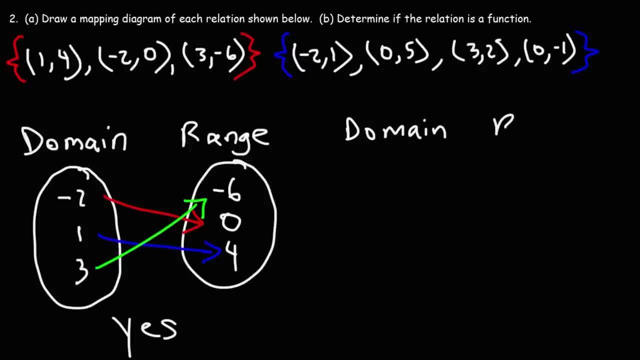 So let's create a mapping diagram as well. So let's start with the domain. The lowest x value is negative 2.. Next we have 0. And then the last one is 3.. Now, looking at the y values, the lowest one is negative 1.. 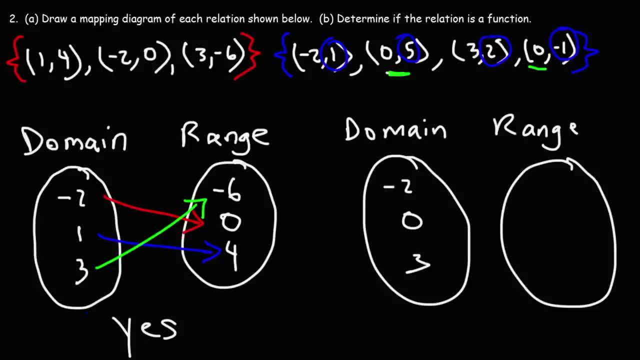 And then it's going to be 1,, 2, and 5.. So negative 2 corresponds to positive 1. 0 corresponds to 5.. 3 corresponds to 2. And 0 corresponds to 2.. 0 corresponds to negative 1.. 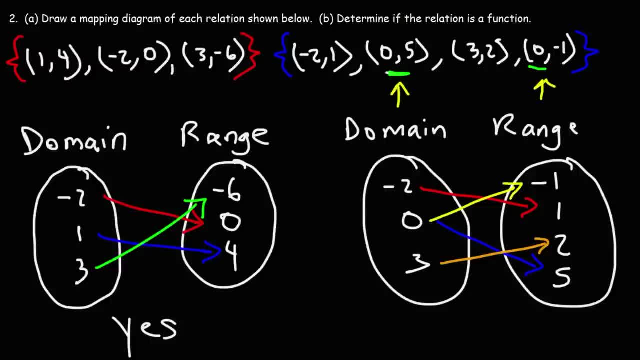 So just by seeing the repeat x values that we see here, we can tell that this is not going to be a function. The two x values have two different y values. You can see 0 points to negative, 1 and 5.. So the second relation is not a function. 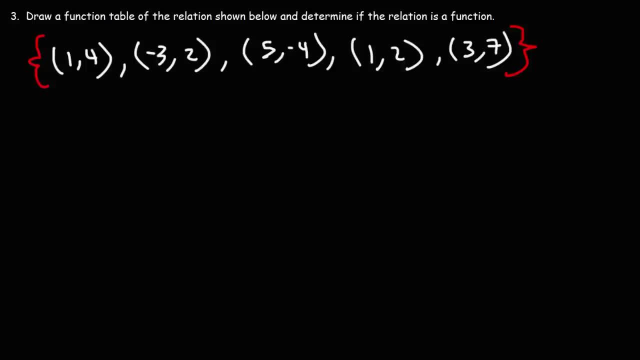 Now for this one. what we're going to do is we're going to draw a function table of the relation And then we're going to determine if the relation is a function. So in this table we're going to list the input values next to the output values. 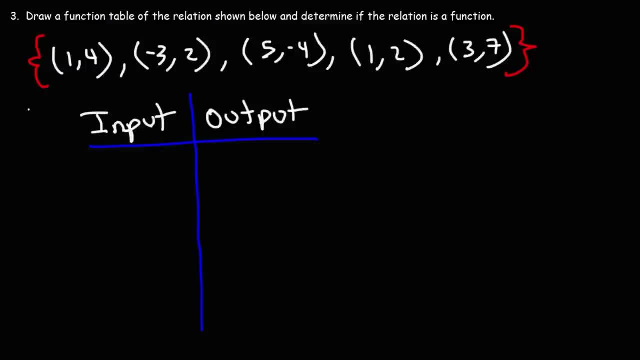 The input values represent the x values. the output values represent the y values. So the input values correspond to the output values, The output values correspond to the domain And the output values correspond to the range. So the lowest input value that we have is negative 3.. 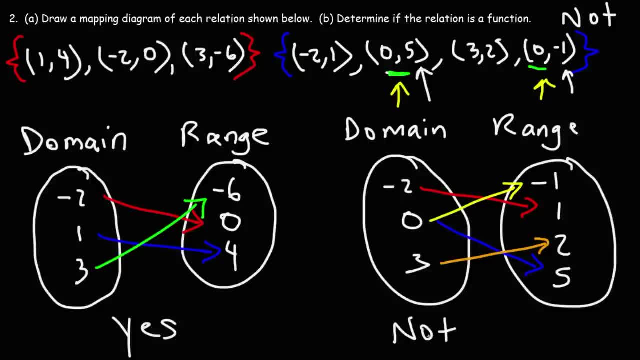 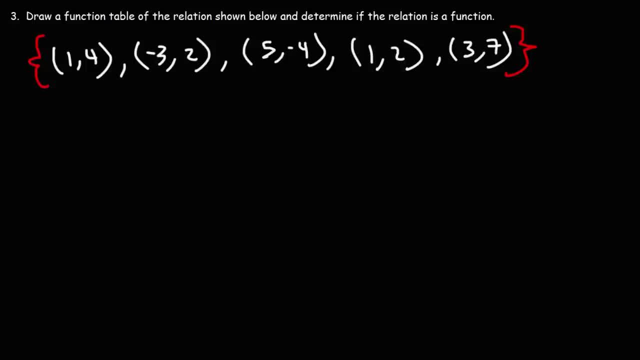 So the second relation is not a function. Now for this one, what we're going to do is we're going to draw a function table of the relation And then we're going to determine if the relation is a function. So in this table we're going to list: 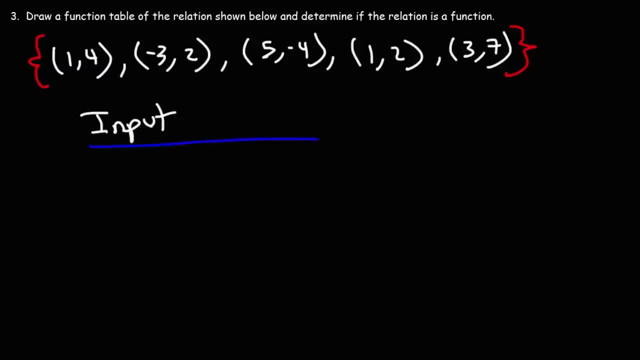 We're going to list the input values next to the output values. The input values represent the x values, The output values represent the y values. So the input values it corresponds to the domain And the output values corresponds to the range. So the lowest input value that we have is negative 3.. 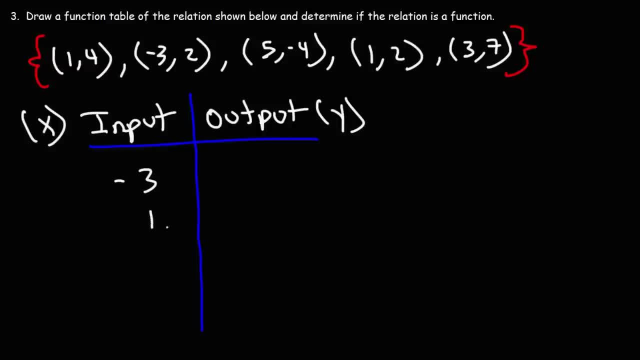 Next is 1.. And then we have another 1. And then, after that is, It's 3 and 5.. Now for this function table. I'm going to write the input value twice, because that's what we have here. 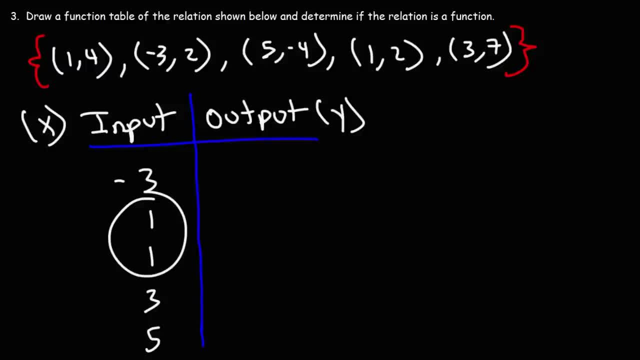 When writing out the domain and the range for repeat values, we would write repeat values once Now. negative 3 corresponds to 2.. For the table, these numbers need to match, So I'm not going to list the output values in a second order. 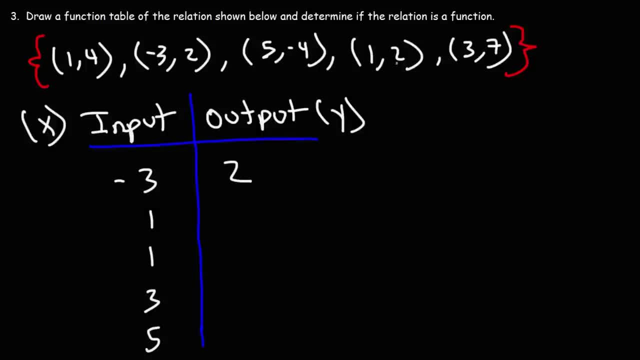 Now for this one. we could use either one, So I'm going to use 1,, 2 for the next one and then 1, 4.. Now when x is 3,, y is 7. And when x is 5,. 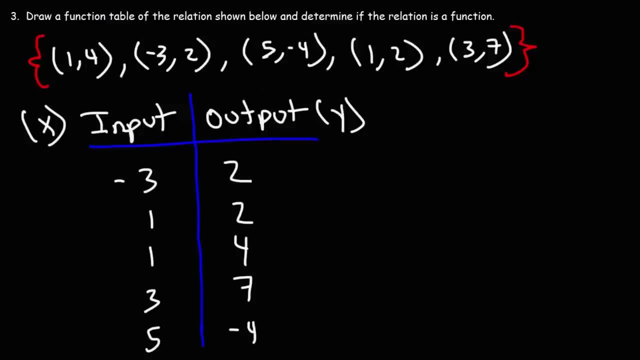 y is negative 4.. So that's the function table, And because we have two identical x values that correspond to two different y values, we know that this relation is not a function. So that's it for this problem. So that's it for this problem. 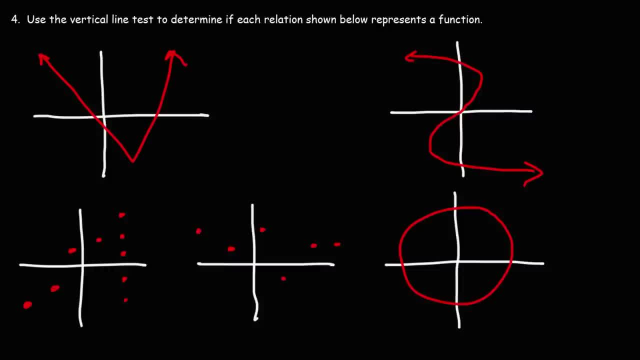 So that's it for this problem. When you have a graph, the best way to determine if the graph represents a function is to use the vertical line test, And that's what we're going to do in this problem. So, any way, you draw a vertical line for the first graph. 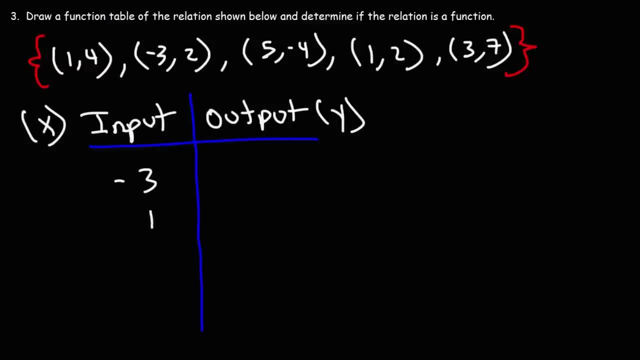 Next is 1.. And then we have another 1.. And then after that is it's 3 and 5.. Now for this function, it's going to be negative 1.. And then after that is it's 3 and 5.. Now for this function, it's going to be negative 1.. 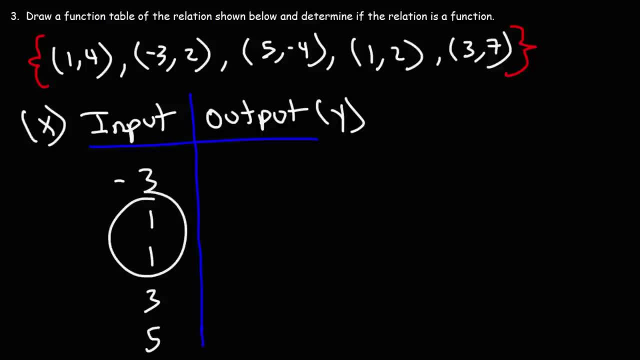 So for this function table, I'm going to write the input value twice, because that's what we have here. When writing out the domain and the range for repeat values, we would write repeat values once Now. negative 3 corresponds to 2.. 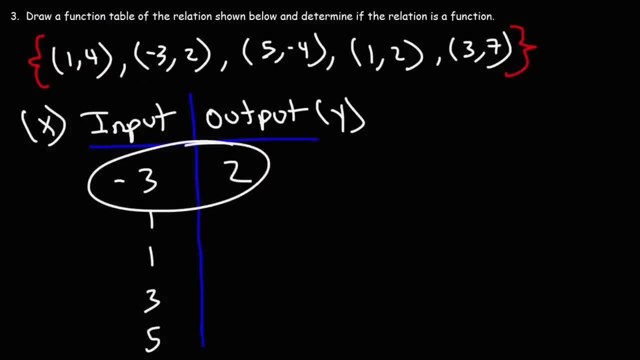 For the table. these numbers need to match, So I'm not going to list the output values in a sudden order. Now for this one, we could use either one, So I'm going to use 1, 2 for the next one, and then 1, 4.. 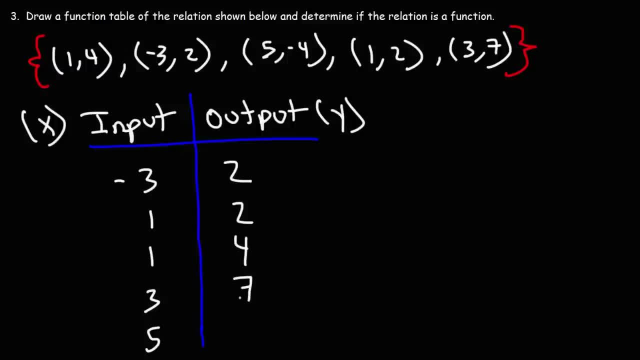 Now, when x is 3, y is 7. And when x is 5, y is negative, 4.. So that's the function table, And because we have two identical x values that correspond to two different y values, we know that this relation is not a function. 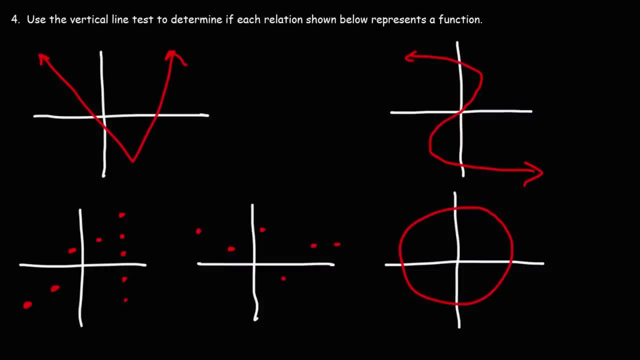 So that's it for this problem. When you have a graph, the best way to determine if the graph represents a function is to use the vertical line test, And that's what we're going to do in this problem. So, any way, you draw a vertical line for the first graph. 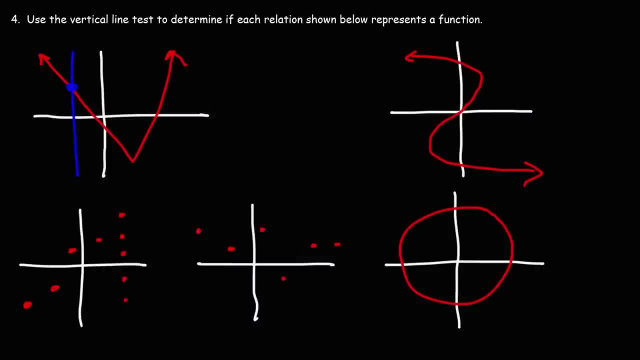 notice that the line only touches the graph at one point. Therefore, the answer is yes, it represents a function For the next one on the right. if we draw a vertical line, notice at this point or place a line at that location. 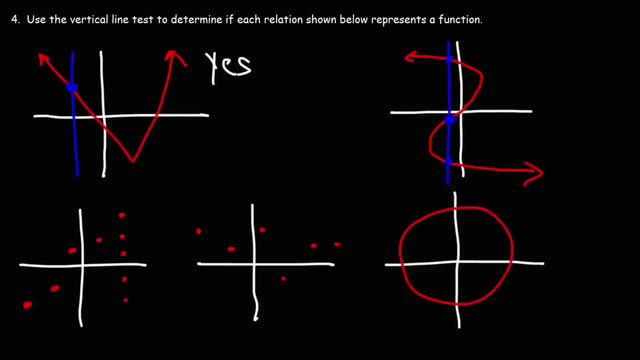 we have three points of intersection between the graph and the vertical line. If we can get two or more points on a vertical line, then the relation is not a function. so we're going to say no. Now if we put the vertical line here. 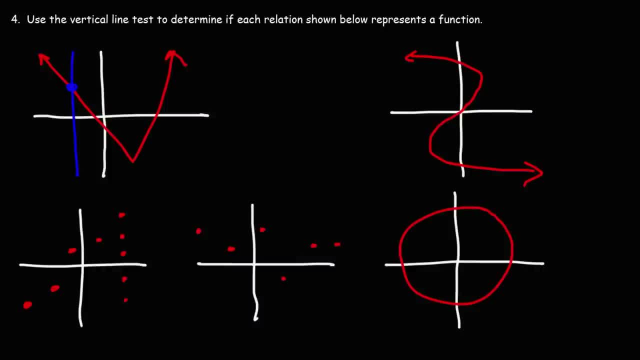 notice that the line only touches the graph at one point. Therefore, the answer is yes, it represents a function For the next one on the right. if we draw a vertical line, notice at this point or place a line at that location. 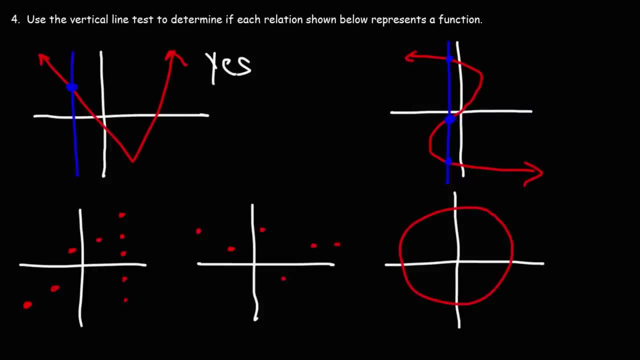 we have three points of intersection between the graph and the vertical line. If we can get two or more points on a vertical line, then the relation is not a function. So we're going to say no. Now if we put the vertical line here. 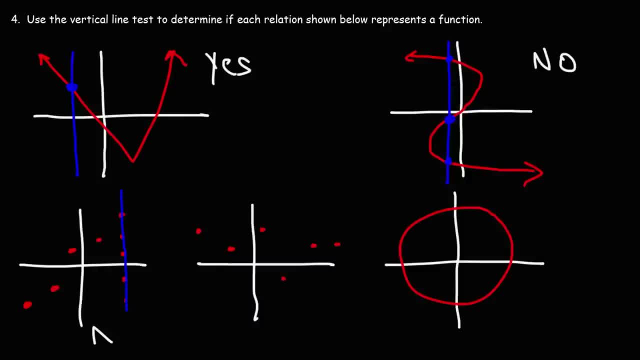 notice that we have five points on that line. So this relation is not a function For the next relation. it doesn't matter where we put the graph, We will only get. I mean, it doesn't matter where we put the vertical line. 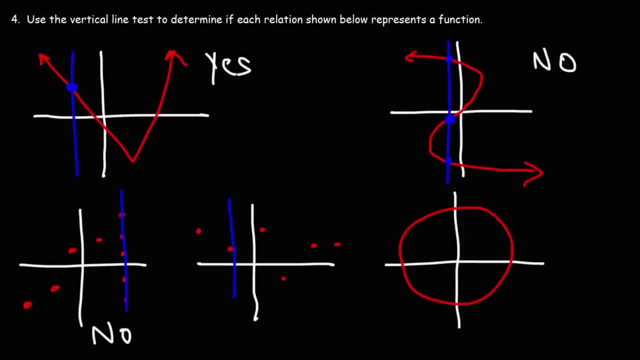 We're only going to get one point If we put it here. it's only going to touch the line once, So we can't draw a vertical line where it touches two points. Therefore, this relation represents a function For the circle. 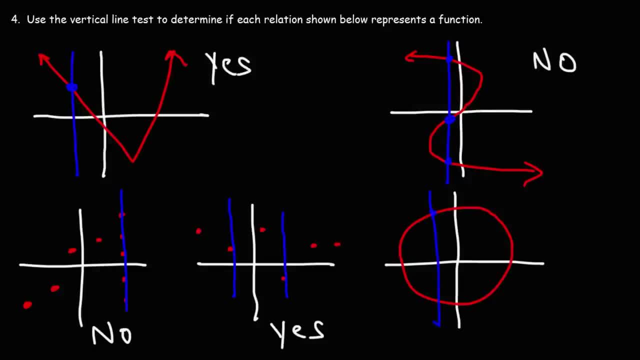 if we put the line here, we can get two points of intersection. So we're going to say yes, I mean no, not yes. This is no. The circle does not represent a function. It does not pass the vertical line test. 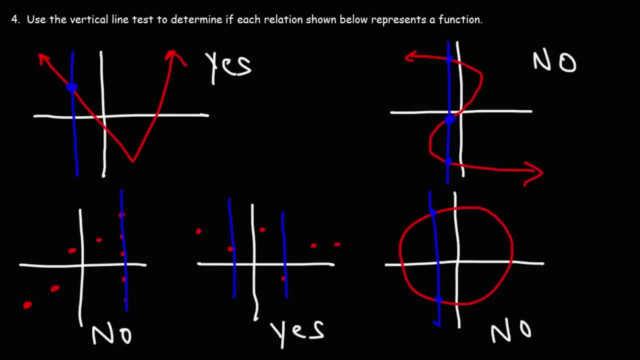 It touches the line at two points. In order for it to pass the vertical line test, the graph must touch the line only at one point, As we saw in these two cases. So that's how you can use the vertical line test to determine if a relation represented by a graph is a function. 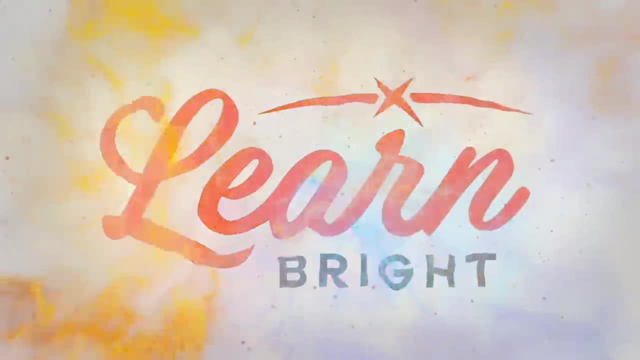 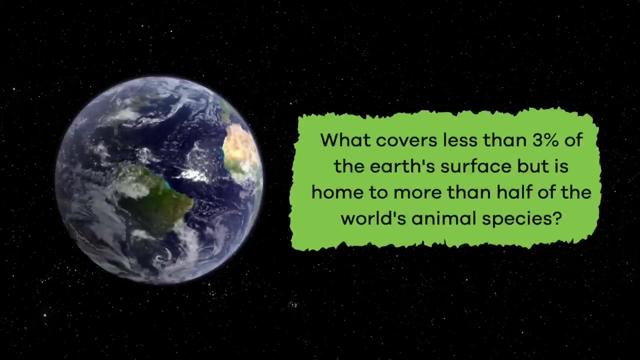 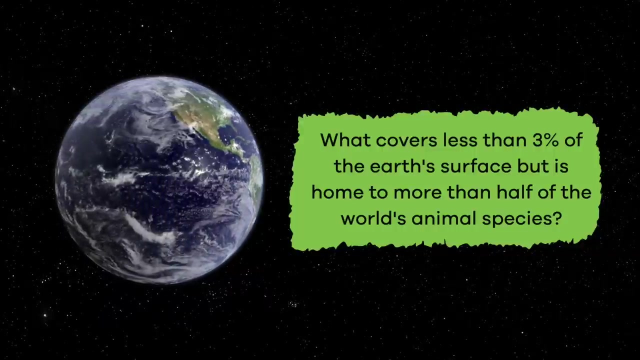 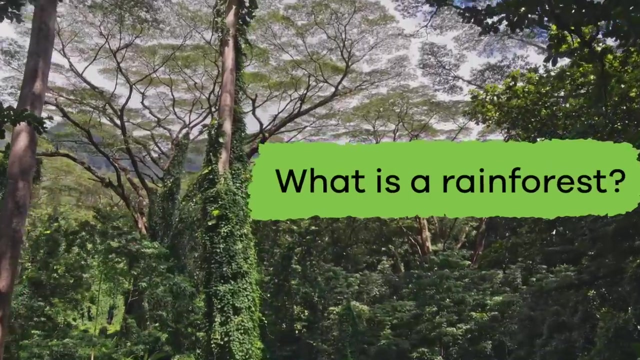 Rainforests for Kids. What covers less than 3% of the Earth's surface but is home to more than half of the world's animal species? Rainforests. What is a rainforest? A rainforest is a thick jungle which is warm.